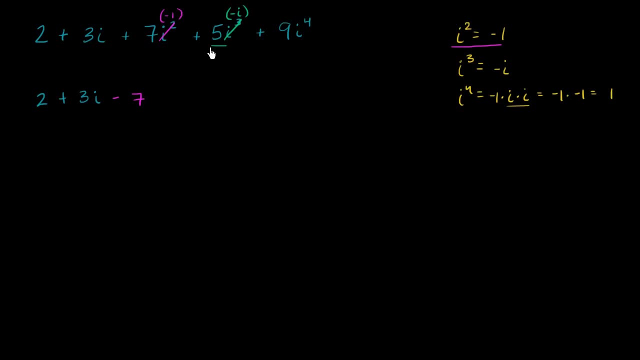 This could be rewritten as negative i, So this term right over here we could write as minus 5i or negative 5i, depending on how you want to think about it. And then finally, i to the fourth. power is just 1.. 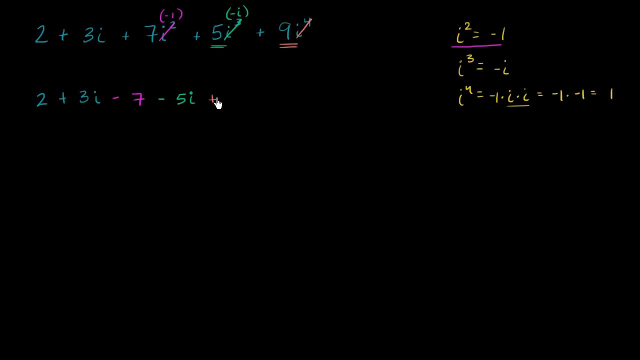 So this is just equal to 1.. So this whole term just simplifies to 9.. So how could we simplify this more? Well, we have several terms that are not imaginary, that they are real numbers. For example, we have this: 2 is a real number. 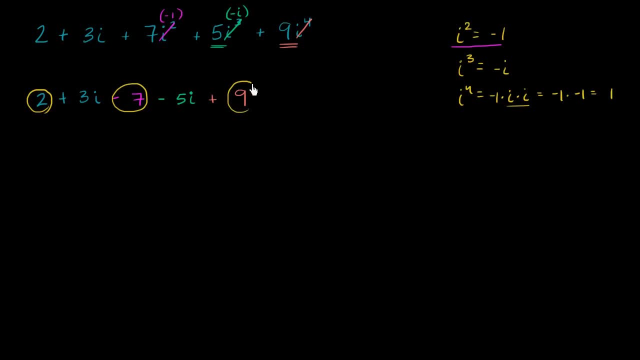 Negative 7 is a real number And 9 is a real number, So we could just add those up. So 2 plus negative 7 would be negative 5.. Negative 5 plus 9 would be 4.. So the real numbers add up to 4.. 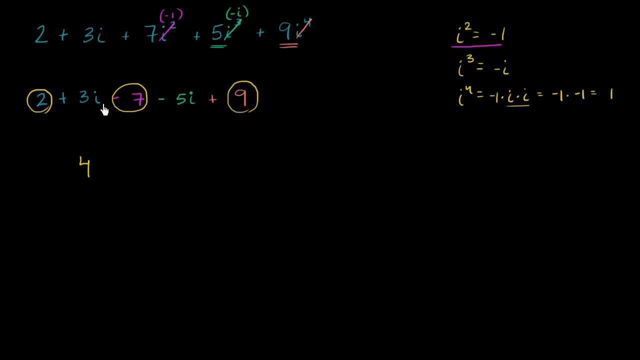 And now we have these imaginary numbers. So 3 times i minus 5 times i. So if you have 3 of something and then I were to subtract 5 of that same something from it, now you're going to have negative 2 of that something. 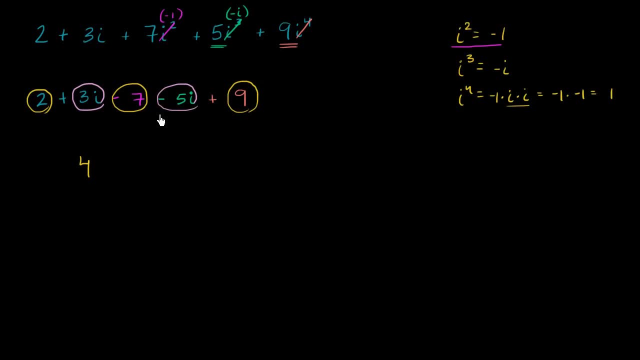 So another way of thinking about it is the coefficients. 3 minus 5 is negative 2.. So 3i's minus 5i's, that's going to give you negative 2i. Now you might say: well, can we simplify this any further? 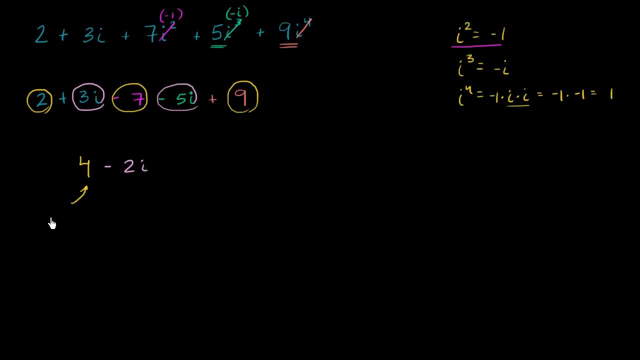 Well, no, you really can't. This right over here is a real number. 4 is a number that we've been dealing with throughout our mathematical careers, And negative 2i, that's an imaginary number, And so what we really consider this is this: 4 minus 2i. 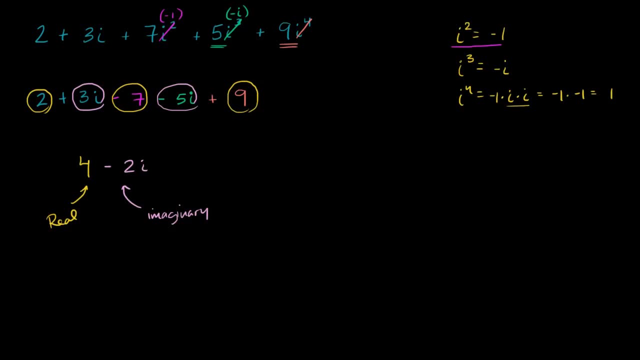 we can now consider this entire expression to really be a number. So this is a number that has a real part and an imaginary part, And numbers like this we call complex numbers. And why is it a complex number? Why is it complex? Well, it has a real part and an imaginary part. 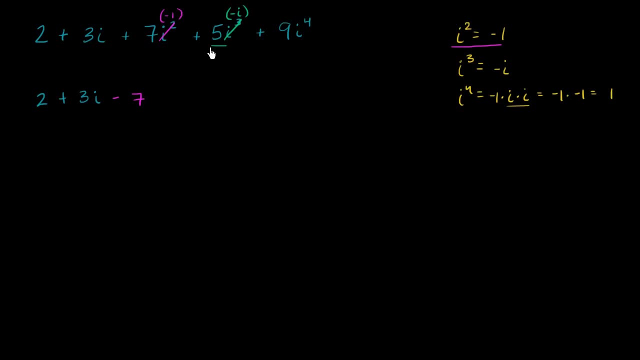 This could be rewritten as negative i, So this term right over here we could write as minus 5i or negative 5i, depending on how you want to think about it. And then finally, i to the fourth. power is just 1.. 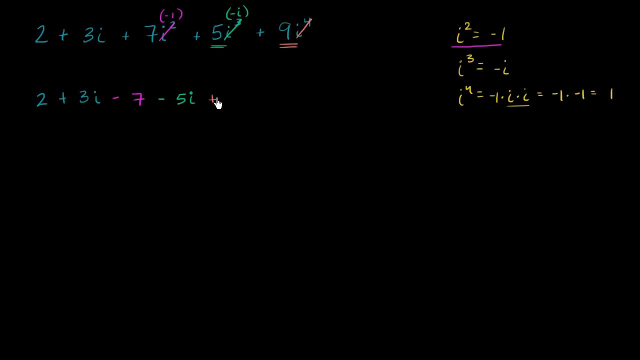 So this is just equal to 1.. So this whole term just simplifies to 9.. So how could we simplify this more? Well, we have several terms that are not imaginary, that they are real numbers. For example, we have this: 2 is a real number. 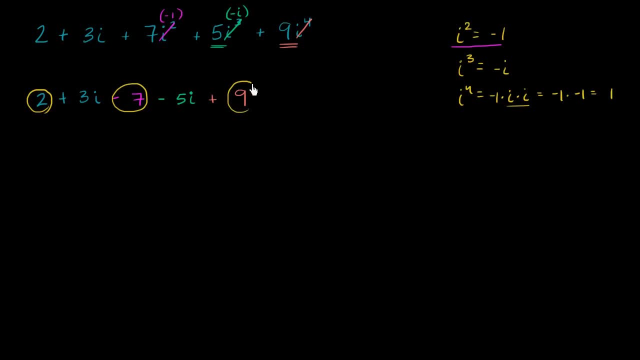 Negative 7 is a real number And 9 is a real number, So we could just add those up. So 2 plus negative 7 would be negative 5.. Negative 5 plus 9 would be 4.. So the real numbers add up to 4.. 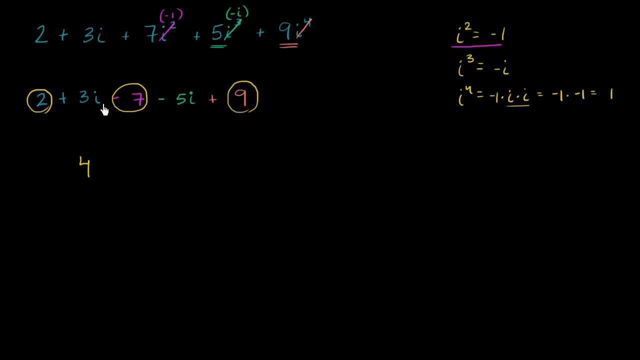 And now we have these imaginary numbers. So 3 times i minus 5 times i. So if you have 3 of something and then I were to subtract 5 of that same something from it, now you're going to have negative 2 of that something. 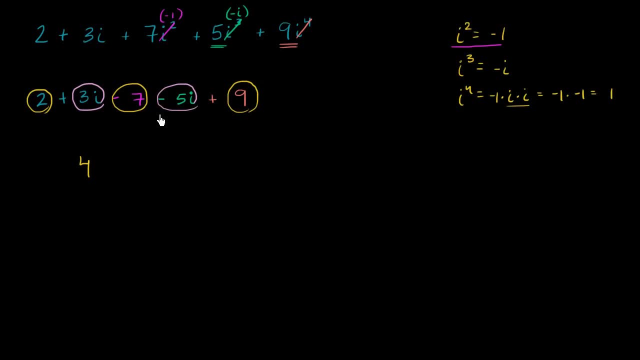 So another way of thinking about it is the coefficients. 3 minus 5 is negative 2.. So 3i's minus 5i's, that's going to give you negative 2i. Now you might say: well, can we simplify this any further? 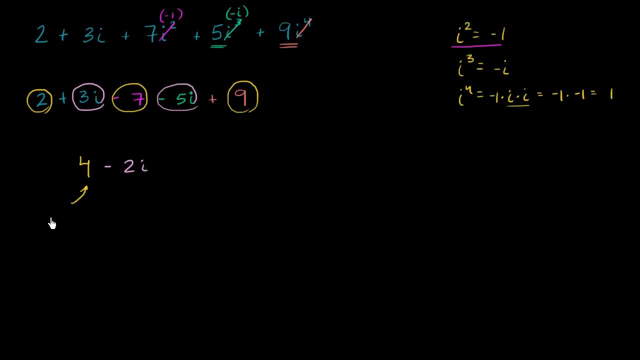 Well, no, you really can't. This right over here is a real number. 4 is a number that we've been dealing with throughout our mathematical careers, And negative 2i, that's an imaginary number, And so what we really consider this is this: 4 minus 2i. 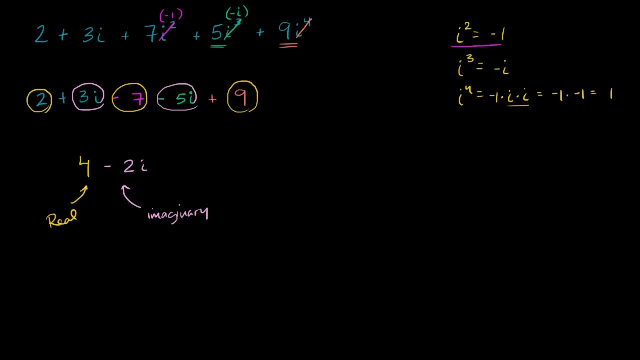 we can now consider this entire expression to really be a number. So this is a number that has a real part and an imaginary part, And numbers like this we call complex numbers. It is a complex number. Why is it complex? Well, it has a real part and an imaginary part.